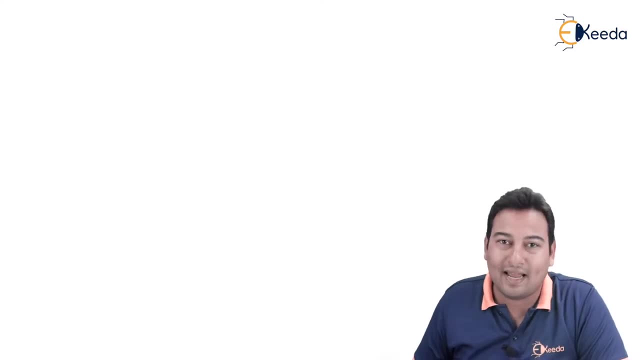 will come in your exam. Let's exactly see what is Gram-Smith method. First of all, you need to know it is used for finding orthonormal basis. Sometimes in the exam it is clearly mentioned Gram-Smith method or it can be asked to find orthonormal basis. 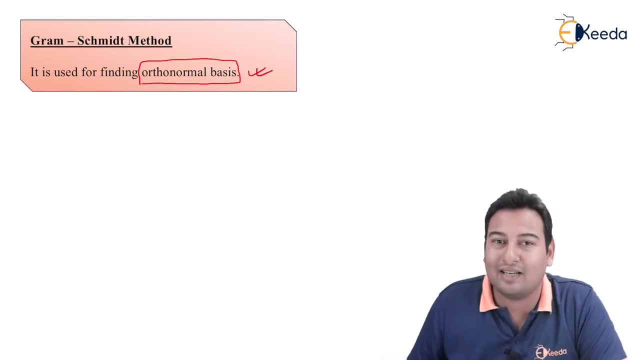 If it is asked to find orthonormal basis, then you should understand it is Gram-Smith method. What needs to be done? Very simple friends. U1, U2 and U3 will be given to you. Three vectors will be given to you. 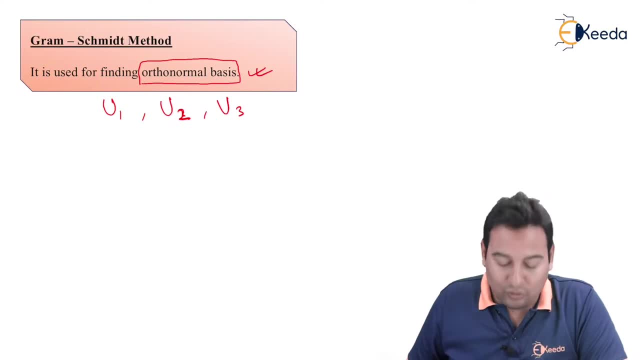 Our aim is to find their orthonormal basis. Orthonormal basis means this is provided to us and we need to find it out. V1,, V2 and V3.. This is our aim. There are formulas for finding V1, V2, V3 that we'll discuss here. V1 is simply U1.. 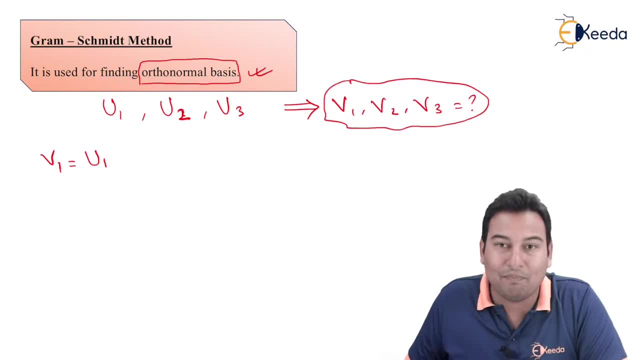 Vector. we already got it. V1 will be simply U1.. V2 will be, see the technique, U2 minus and if it is V3, it will be U3 minus. This will be projection of U2 on V1, because we are talking. 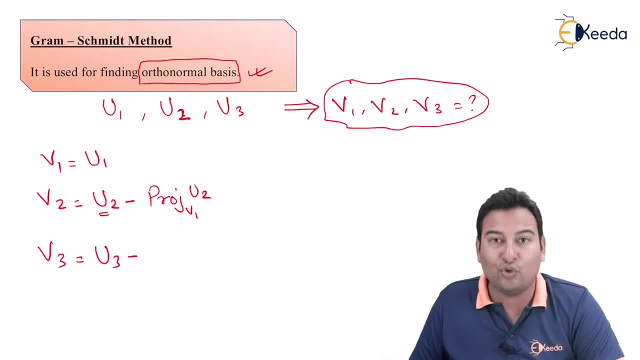 about V2.. Here it is U2, U2 on previous, that is V1.. Here it will be projection of. we are talking about U3.. So U3 on V1 minus projection of U3, and the previous is V1 and V2 both. Therefore, we are going to take projection of U3 on V1. 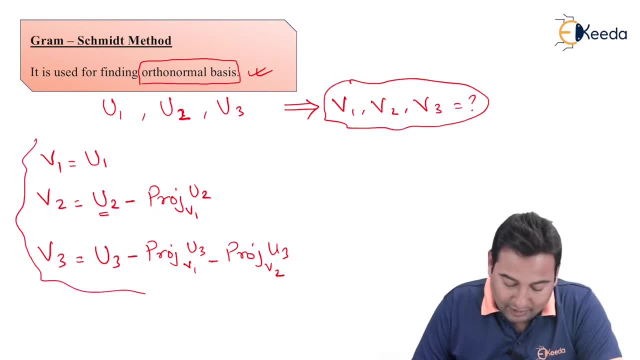 and projection of U3 on V2.. These are the formulas. In the last video we discussed how to find the product projection. Now we'll see example on it. This is the most common example of projection of U3 on V2.. So we are going to take projection of U3 on V1 and projection of U3 on V2.. 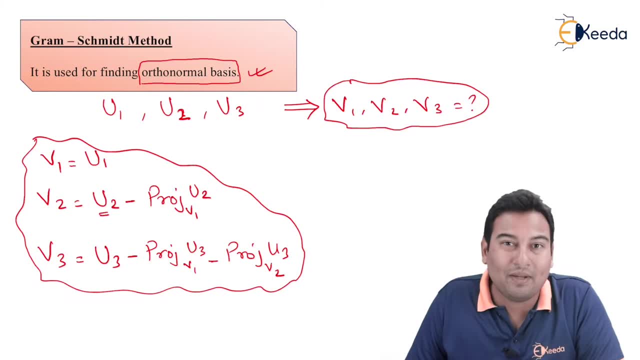 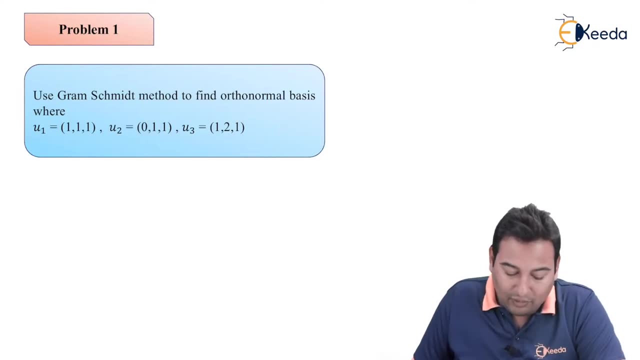 This is the most important part of vector spaces. If you understand this topic, you can confirm your marks in the exam. Let's start with the first: U1, U2 and U3. all are given to us. We need to find it out V1, V2 and V3.. Use Gram-Smith method to find orthonormal. 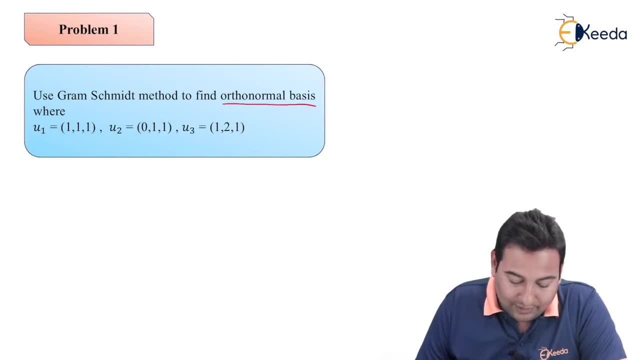 basis. First of all, as discussed, see here, V1, V2, V3 want. V1 is directly U1. So V1 is directly U1. That's it. We got V1 as 1, 1 and 1.. First part is done. Next we need: 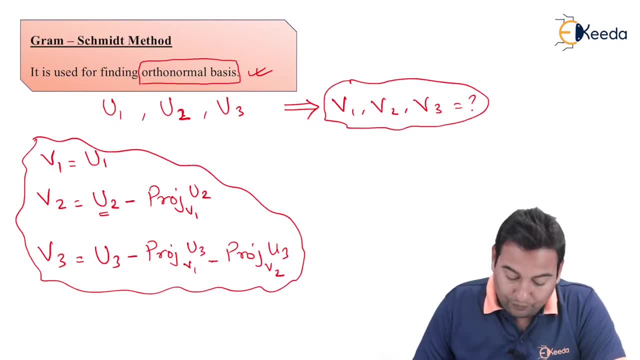 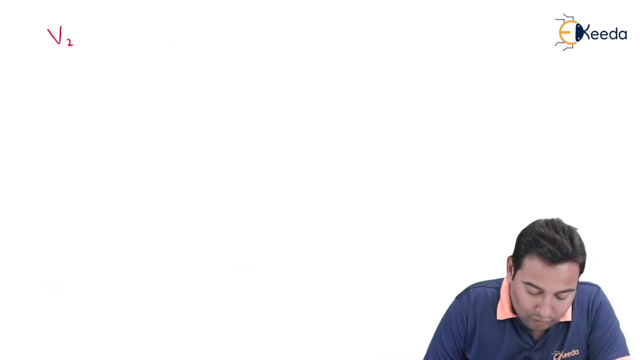 to find it out: V2.. For V2, we want this particular term, That is, projection of U2 on V1. V2 is U2 minus projection of U2 on V1.. Here, U is small, Therefore we need to take small. 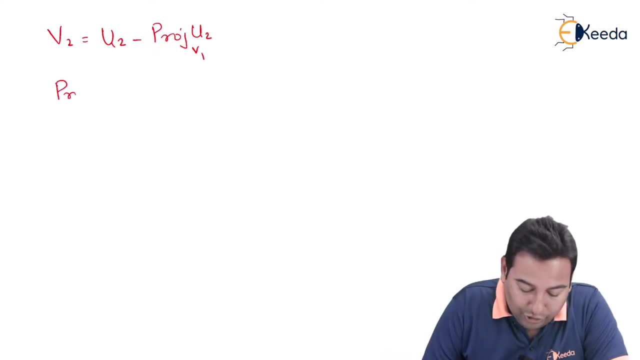 First of all, we will find it out: projection of U2 on V1.. Then we are going to put and we are going to get the value of V2.. As discussed, this is U2 dot, V1 dot, product of both divided. 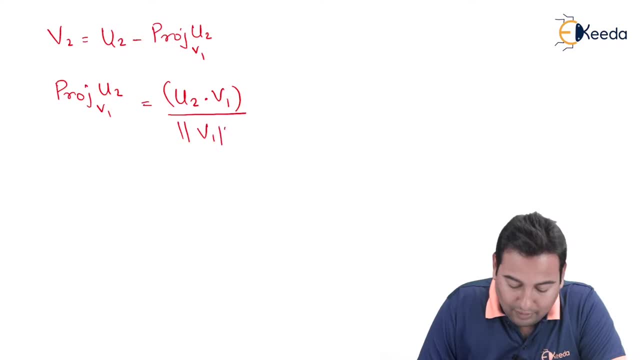 by norm of V1, the whole square dot V1.. U2 dot, V1 dot. product of U2 and V1.. V1 is 1, 1, 1 and U2 is 0, 1, 1.. Let me write it down here for reference: V1 is 1, 1, 1 and. 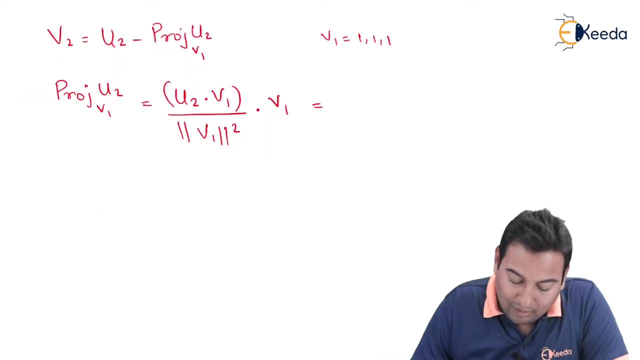 U2 is 0, 1, 1.. This is for reference. Let's find it out there: dot product U2, dot V1.. That is 0 plus 0.. V1 is 1, 1 and 1. the whole divided by norm of V1, the whole square. The whole square means: 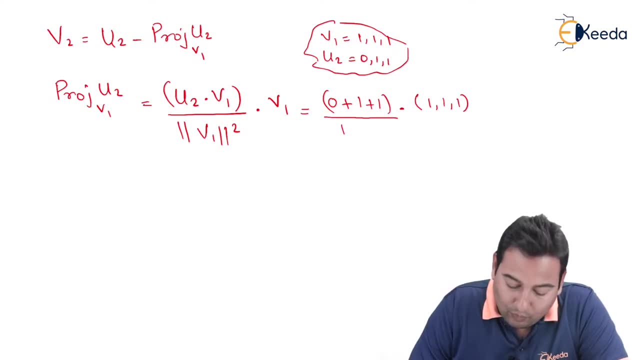 square, root and square will be cancelled. We'll get 1 plus 1 plus 1.. That will be 2 by 3, and inside we have 1, 1, 1.. Let's multiply: inside, We will get 2 by 3, 2 by 3 and 2 by. 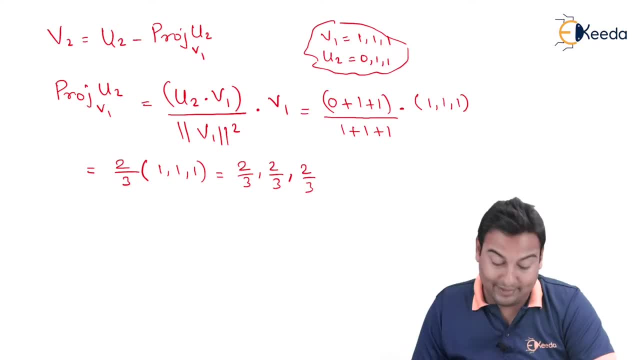 3. 3. if we multiply 2 by 3 inside, this is projection of u2 on v1. my aim is to find v2 c here. that is u2 minus projection of u2 on v1. u2 we already know. that is 0, 1, 1 minus projection of u2 on v1. 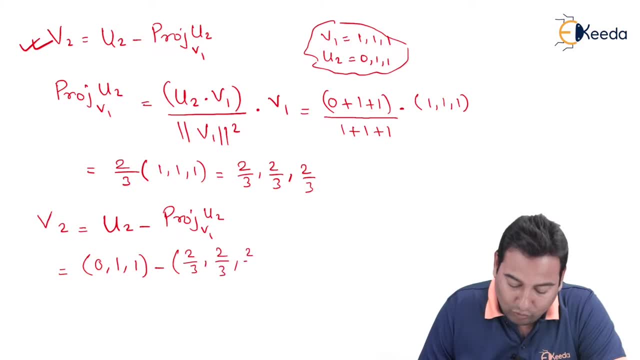 that is 2 by 3, 2 by 3 and 2 by 3. if we solve, we'll get v2, as just need to subtract: 0 minus 2 by 3 is minus 2 by 3. 1 minus 2 by 3 is 1 by 3, and 1 minus 2 by 3 is 1 by 3. this is v2. 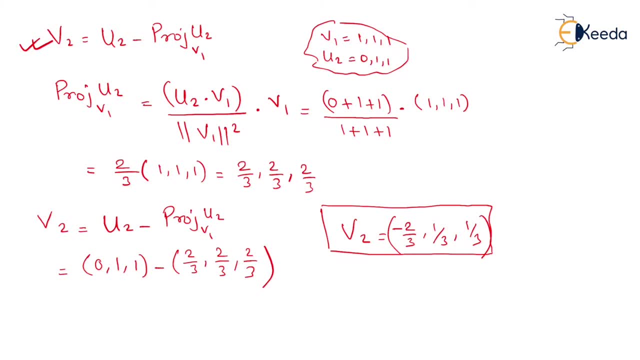 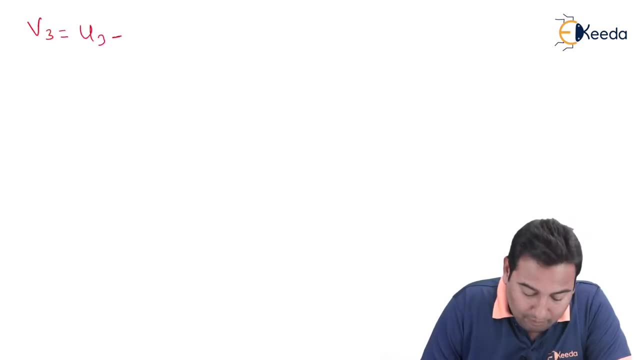 we got v1, we got v2. we need to find it out v3. now for v3, the formula is very simple: u3 minus projection of u3 on both previous, that is, v1, and projection of u3 on v2. for finding v3, we want these two projection. let's find it out that projections. 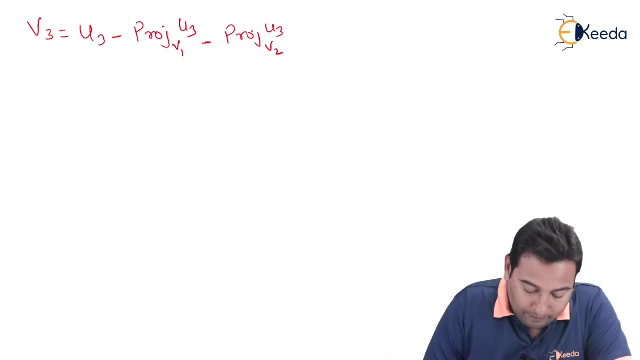 for reference. we want v1, which is 1, 1, 1. we want v2- we got it as minus 2 by 3, 1 by 3 and 1 by 3. also, we want u3. u3 is 1, 2 and 1. this is v1, v2 and u3. let's find it out. the projections. 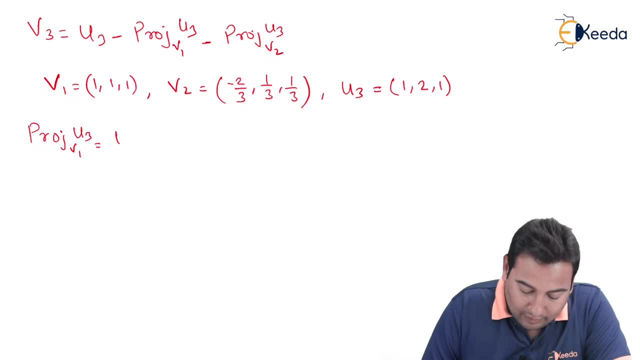 u3 on v1, that is u3 dot, v1, it's dot product, v1 upon norm of v1, the whole square, which will be equal to u3 dot. v1, it's dot product of v1 and u3, that will be 1 plus 2 plus 1 dot. v1, that is 1: 1 and 1 upon 3, which will be equal to. 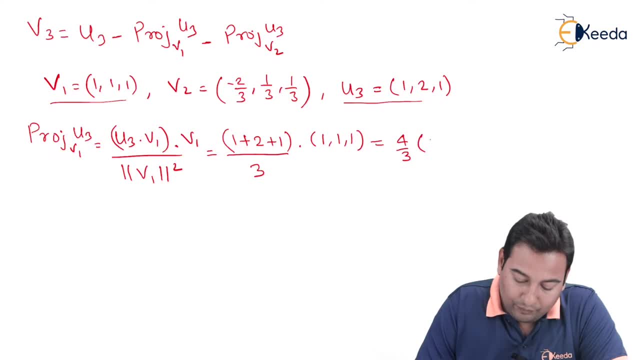 4 by 3, 1, 1, 1. if you multiply 4 by 3, inside that will be 4 by 3, 4 by 3 and 4 by 3. this is projection of u3 on v1. now let's find your projection of u3 on v2. 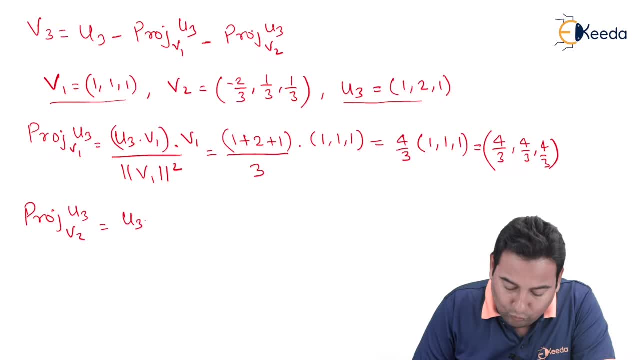 that will be u3 dot v2, v2 upon norm of v2, the whole square, which is equal to u3 dot v2. that means i am going to take its dot product, v2. that is minus 2 by 3 plus 2 by 3 plus 1 by 3 dot V2.. V2 is minus 2 by 3, 1 by 3 and 1 by 3,. 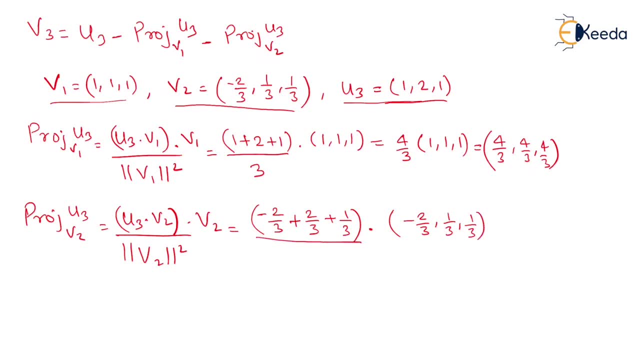 the whole divided by norm of V2 square, that is, 4 by 9,, 1 by 9, 1 by 9.. This will be cancelled. will get 1 by 3 upon 6 by 9 minus 2 by 3, 1 by 3 and 1 by 3, which is equal to 1 upon 3. 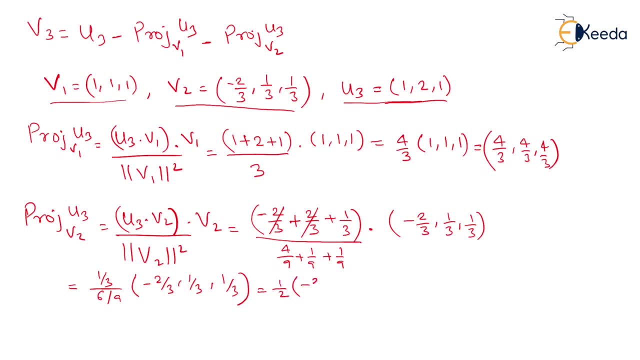 divided by 6 by 9 means 1 by 2, minus 2 by 3, 1 by 3 and 1 by 3.. If this 1 upon 2 goes inside, projection of U3 upon V2 will become minus 1 by 3,. 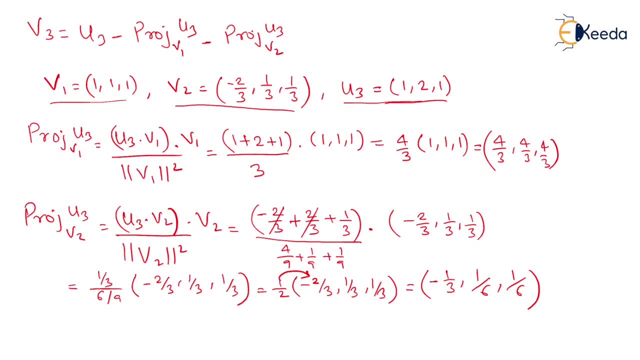 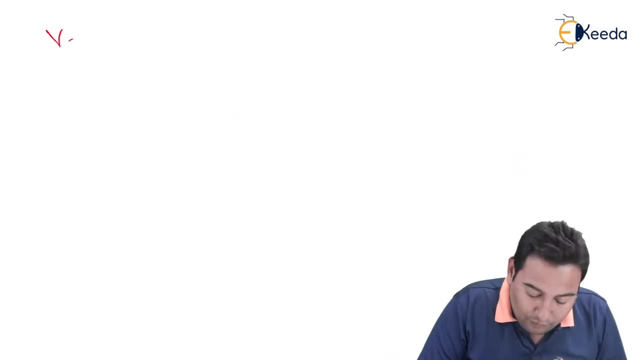 1 by 6 and 1 by 6.. We got both the projection. Let us put in the formula of V3 to get the result: V3 is U3 minus projection of U3 on V1 and projection of U3 on V2.. U3 is 1 to 1. 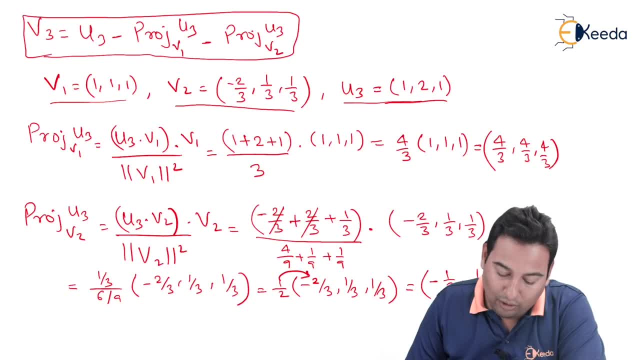 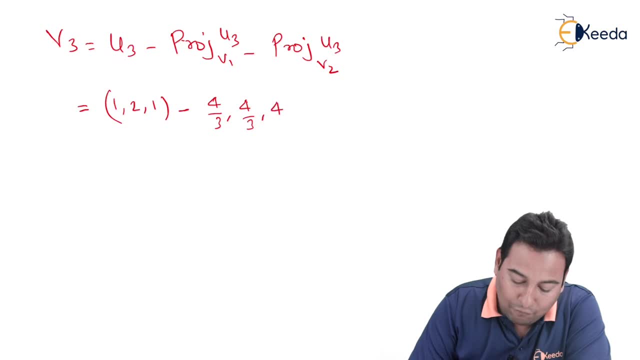 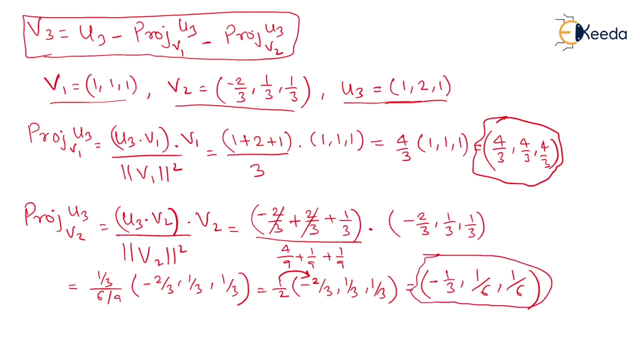 minus projection of U3 on V1.. This is the value That is 4 by 3, 4 by 3 and 4 by 3 minus projection of U3 on V2.. This is the value That is minus 1 by 3, 1 by 6 and 1 by 6.. 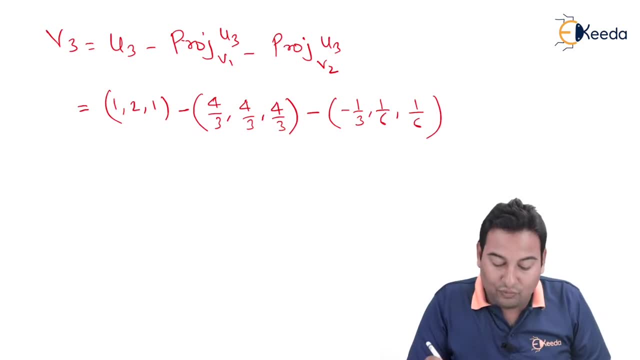 What needs to be done is we need to subtract this First value, that is, 1, minus 4 by 3, and this minus needs to multiply it inside. That means 1 minus 4 by 3, plus 1 by 3 comma, 2 minus 4 by 3, minus 1 by 6 comma 1 minus 4 by 3.